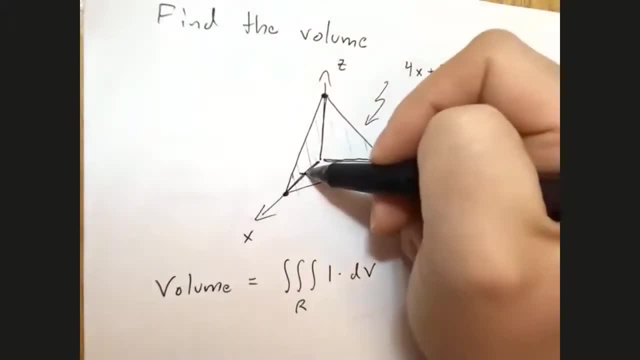 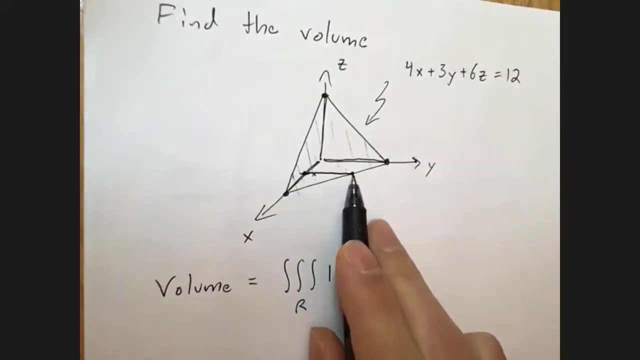 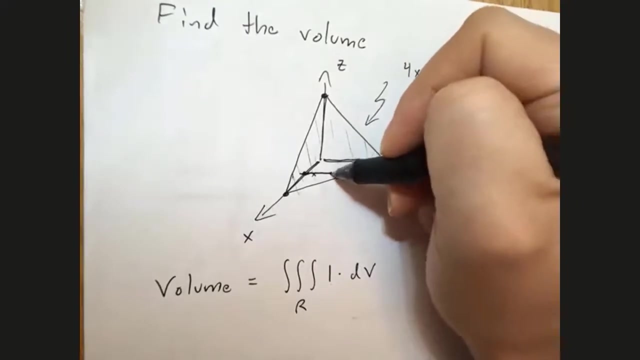 going to integrate here And now, for each x, I'm going to integrate this. I'm going to find I can specify different values of y by integrating in this direction. Right, So for each fixed x, I can let y vary from here to here. Right, And then for each of those y's I can go from here up to the. 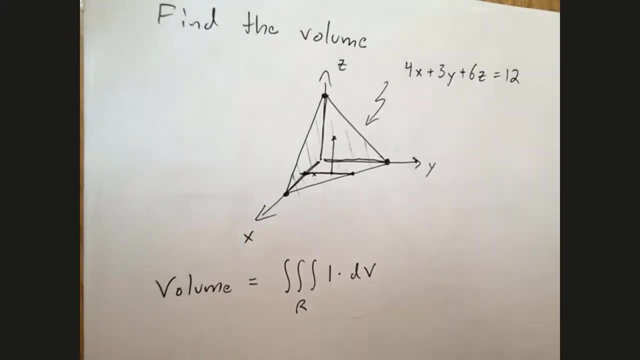 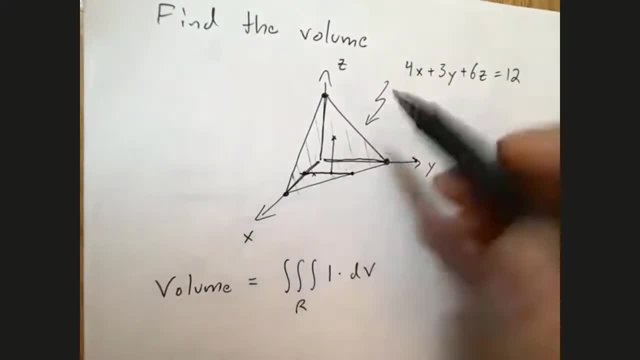 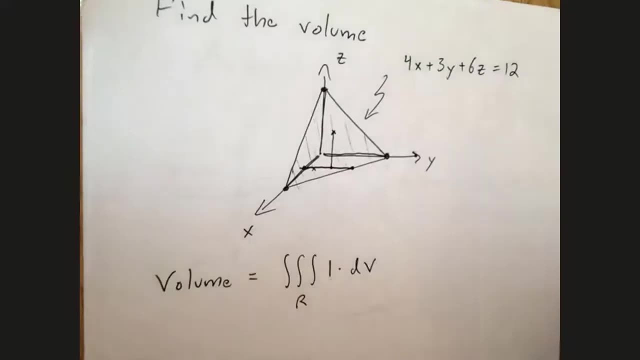 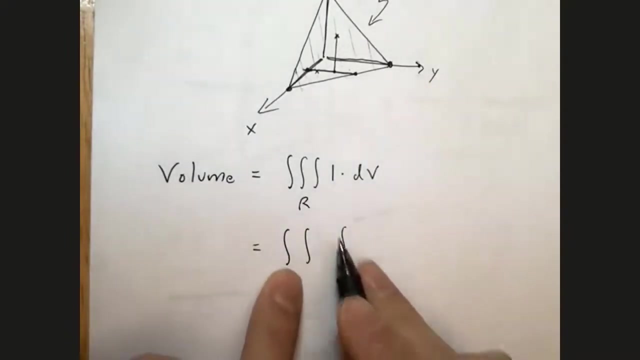 here to here, And then for each fixed x and y, I let z go from here to here, And that will get me through every single point in this tetrahedron. So that's one way to set up this integral We started by. I'm going to leave some space here because I'm going to put some stuff up here. 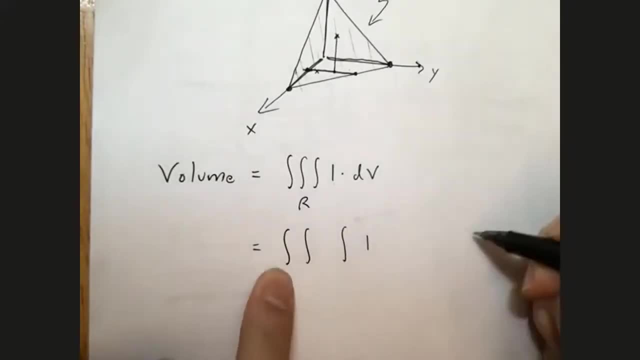 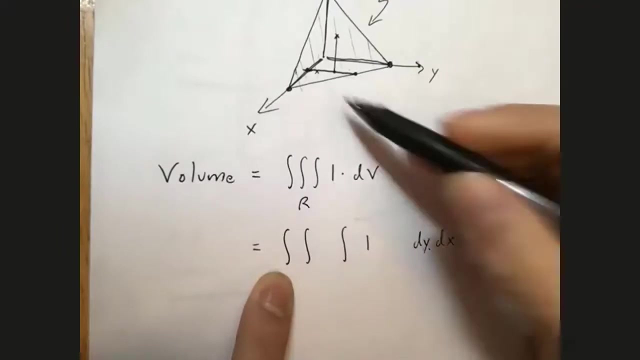 We started by fixing x, So x goes on the outside. And then for every fixed x we integrated in the y direction Right, So y is next, And then for each fixed x and y. once I had those figured out, I got to this point. 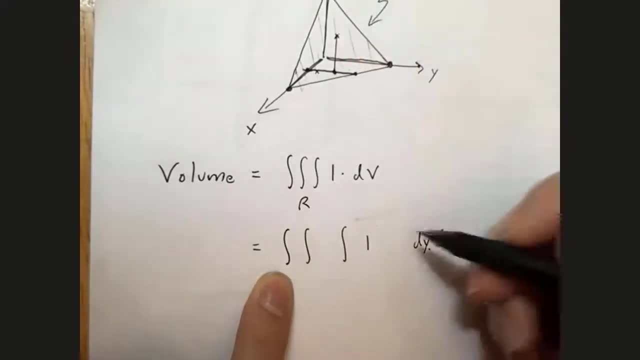 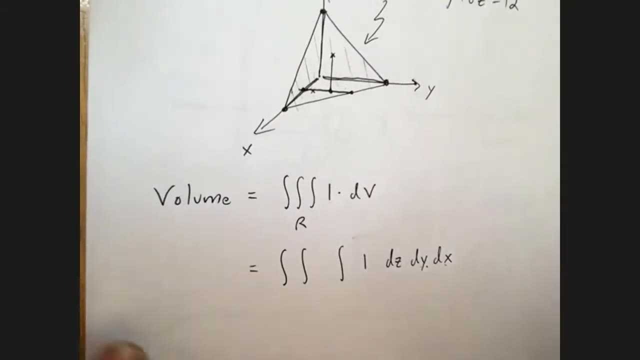 I integrated in the z direction, So z is last. So you work from outside in. Now, what are we going to put in these bounds? Well, x is the easiest. What values of x do I do this for? Well, I just have to figure out where I started from. Well, that's clearly. x equals 0.. 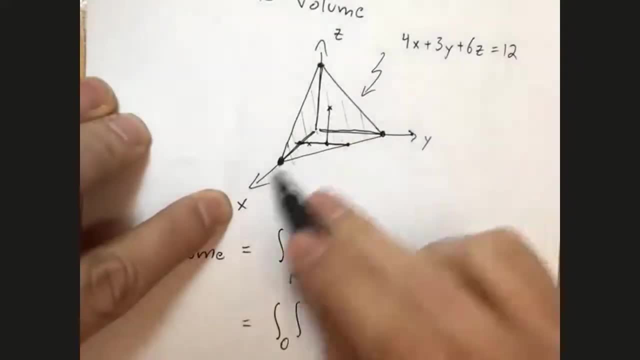 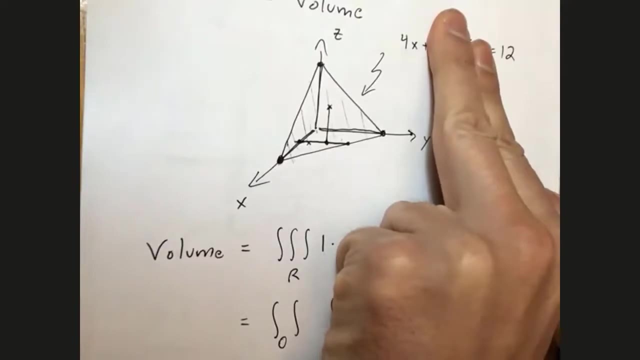 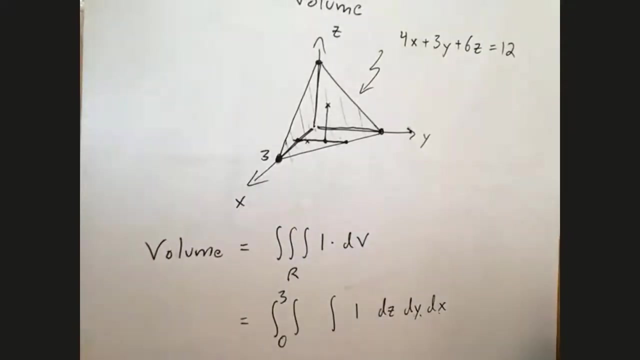 And then I have to figure out where I ended at. Well, I'm on the x-axis, So y and z are 0. So that just says 4x equals 12.. So x must be 3.. So x goes from 0 to 3.. That's the easiest part. 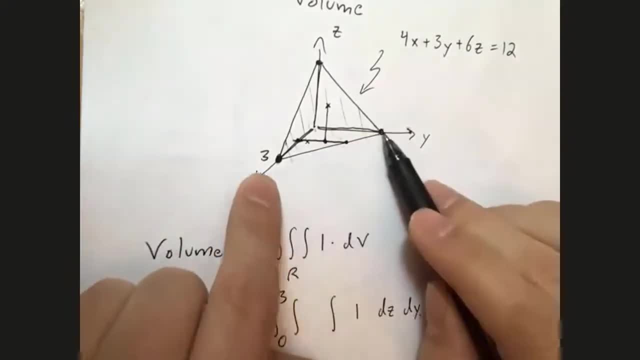 I can also figure out what these points are, Because at this point x and z are 0, so I just solve that equation. I get y equals 4. And this point is when x and y are 0. So that's when z is equal to 2.. 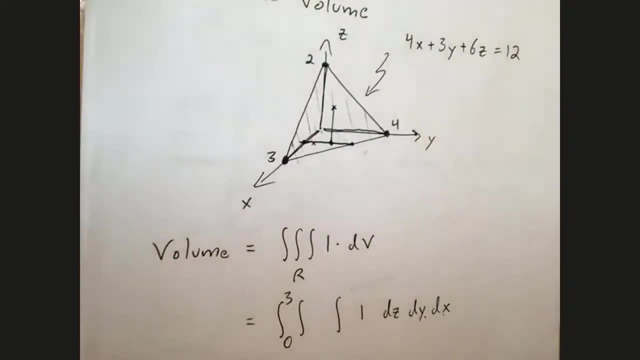 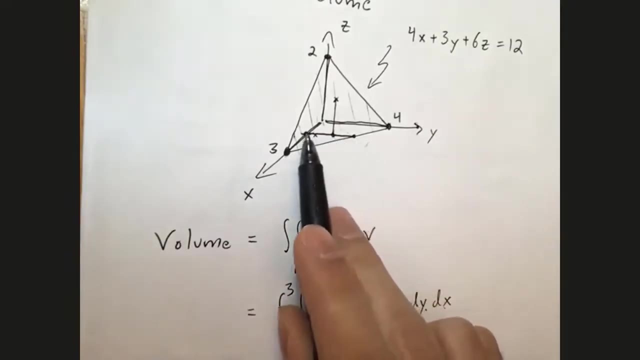 So I can figure out what these these intercepts are. And now I can figure out what the bounds for this integral are. Right, It starts at 0.. y starts at 0.. So I know I can put 0 down there. 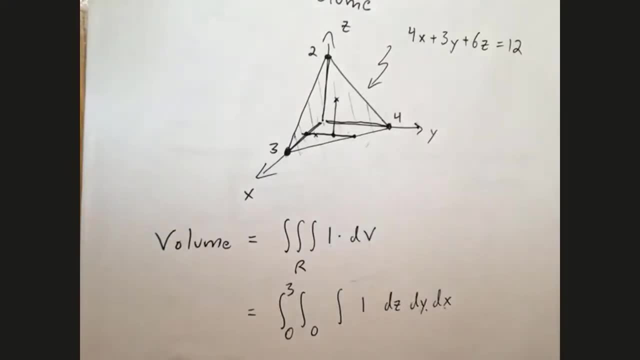 How high does y go? Well, y goes up to this line, All right. Well, this is not going to be a constant right, Because it depends on x. Depending on what the value of x is, I go a different distance. 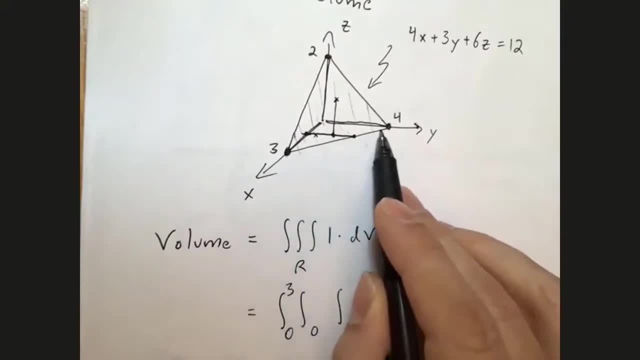 So we have to figure out what function of x. this is Okay, let's figure that out. So let's look at this graph in the xy-plane. So let's just take it down here. So we have x and y, Oops, 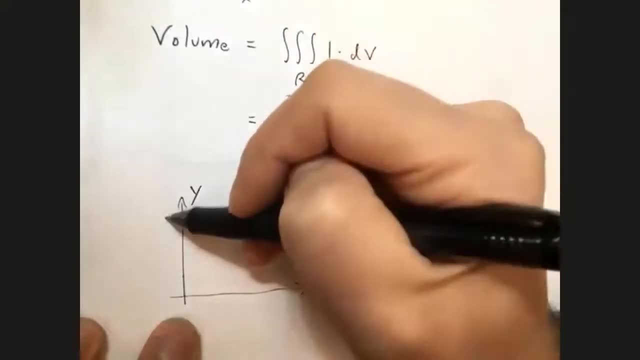 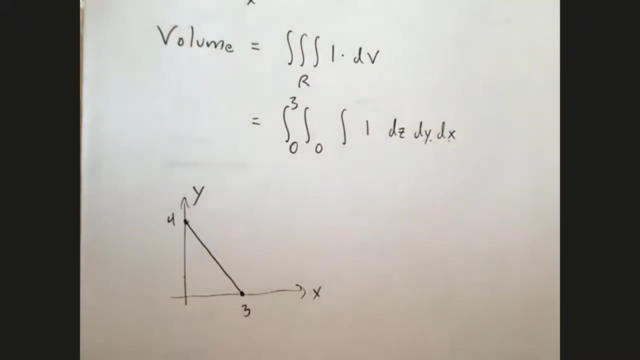 And I'm just going to draw that line. It had y intercept 4 and x intercept 3.. Right, so that was the line that I was looking at. It's the same thing, just looking at it from above in the xy-plane. 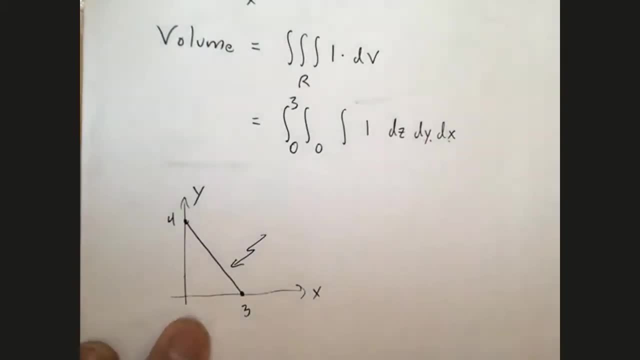 So what function of x is this? Well, this is pretty easy, because it's a straight line, Its slope is negative 4 thirds And its y intercept is 4.. so there it is. so that is what this line is represented by, and that's how high Y. 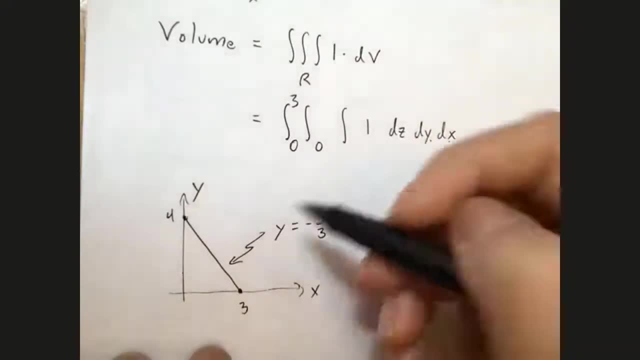 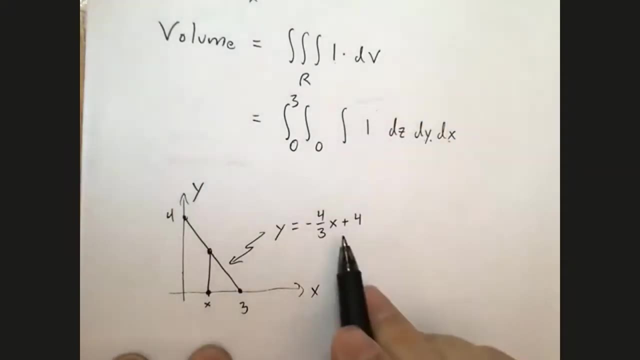 goes. so what I'm doing is I'm really going from. you know, when I fix an X, Y is going from here to here, so it's going up to this height. so that's what I put here: negative 4 thirds X plus 4. now what about the Z? okay, so once I've specified, 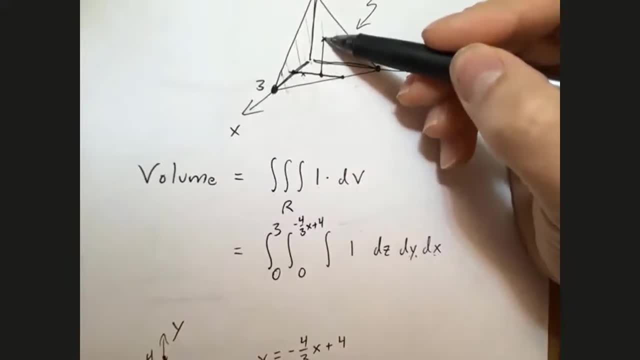 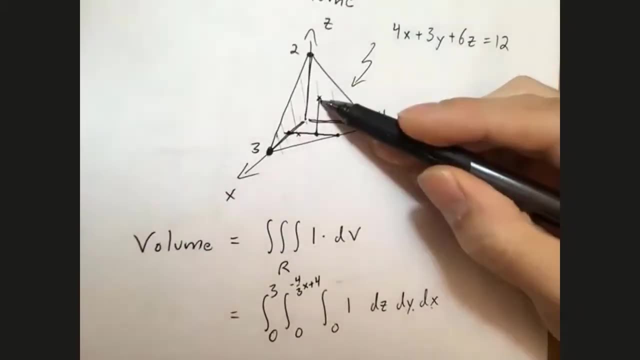 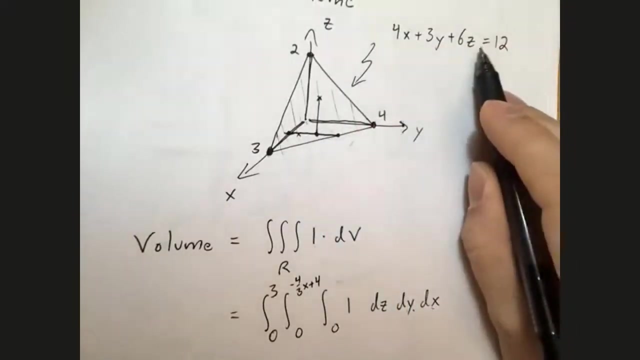 those. I need to see how high to go. well, I'm going to start at 0, that's clear. I start down here. how high do I go up here? well, that's determined by the height of this surface. what's the height of the surface determined by? well, it's here's. 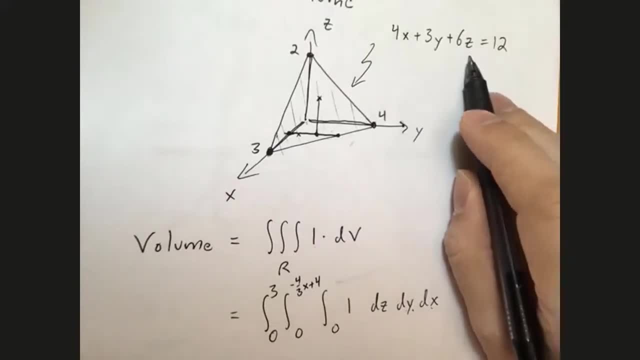 the equation right here. just solve this for Z. so if you solve this for z, then you get the height of the surface and you get the height of the. for Z you get. let's see, we'll subtract these things from both sides and then divide by 6.. 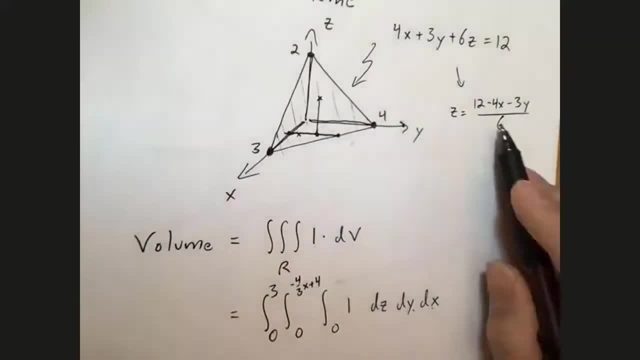 Right, so that's the height that we have to go, So that's the thing that goes over here. All right, so I'm going to have up here. I'm going to have 12 minus 4x minus 3y over 6.. 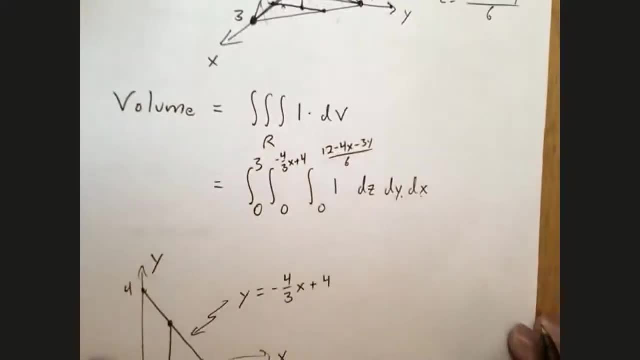 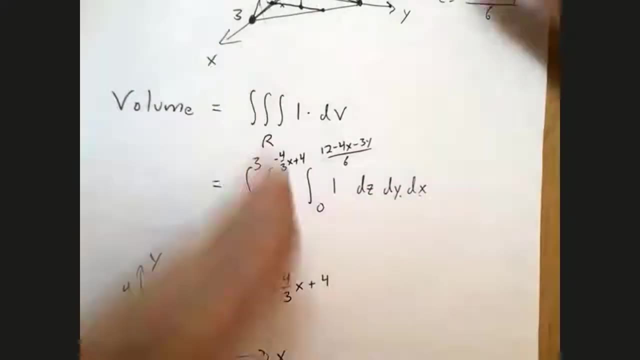 That's, that's the bound, upper bound on the innermost integral, And we can figure out this integral. I'm not going to go through all the steps of figuring out. I see there's fractions. it's probably going to fill up an entire sheet of paper if I try to do it here in big writing, big. 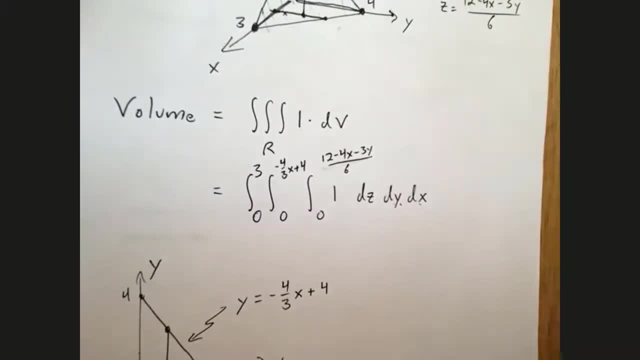 so, for the screens, What I'm going to do, I'm going to go to maple and do it all right. It's not a hard problem because I think these, these functions are just, they're all linear, right. So it's not difficult, it's just it's going to take up. I'm running out of paper over. 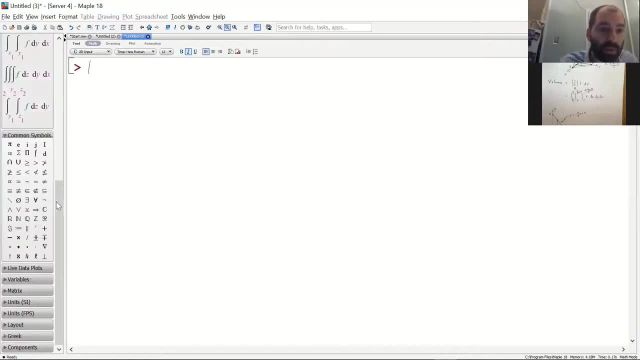 here. So okay, so what was the integral we were doing? Well, we were doing a triple, triple integral, so I'll just grab triple integral of bounds over here. We said that the- oh good, it's even set up in the order that I set it up in. How nice. 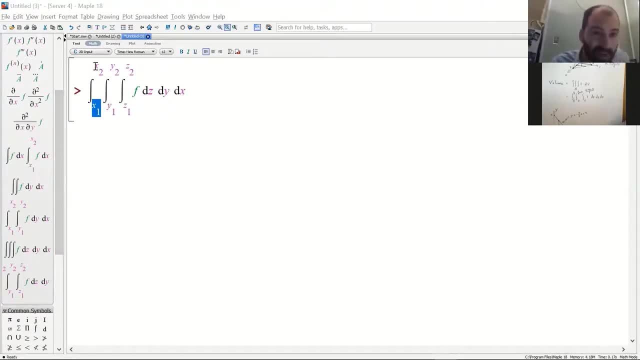 I looked out there, The x went from 0 to 3,, 0 to 3.. The y went from 0 to negative four-thirds x plus 4.. And the z went from 0 to 2.. Then we had that fraction: 12 minus 4x minus 3y, all over 6.. The function that we integrated was: 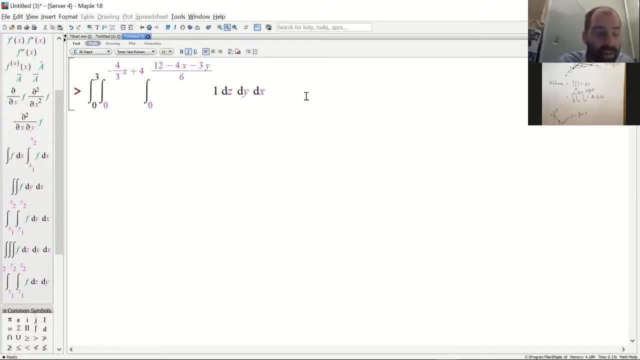 1,. all right, And let's see. make sure that you got dz, dy, dx. You may need to change those orders if necessary, but it's set up right. Oh wow, look at this. Maybe we could have done it by hand if. 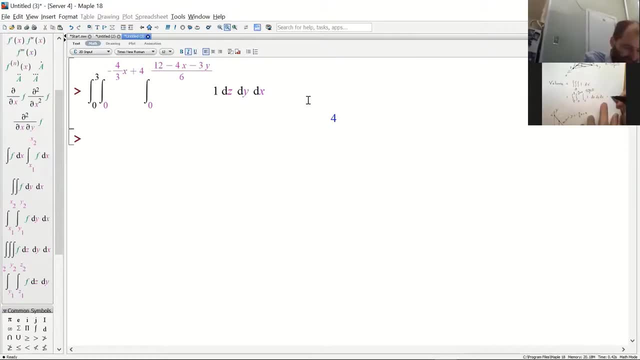 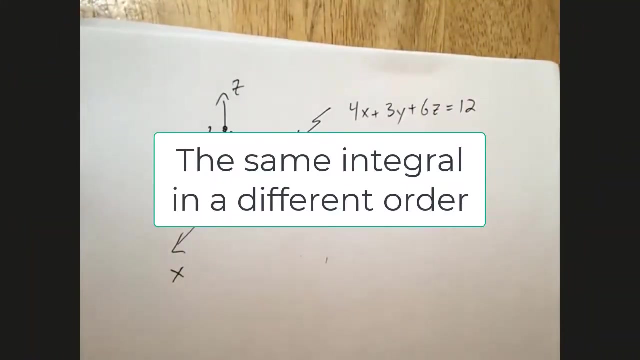 it came out that nice, The answer is just 4.. All right, not too shabby. So I you should, as an exercise, go through and do this by hand. It looks like it'll be pretty, it'll come out all right. So suppose I wanted to do let's really. 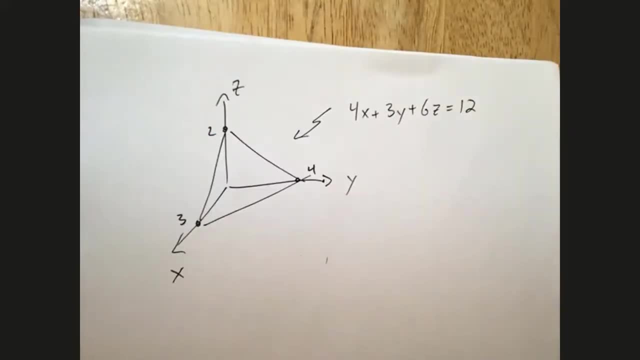 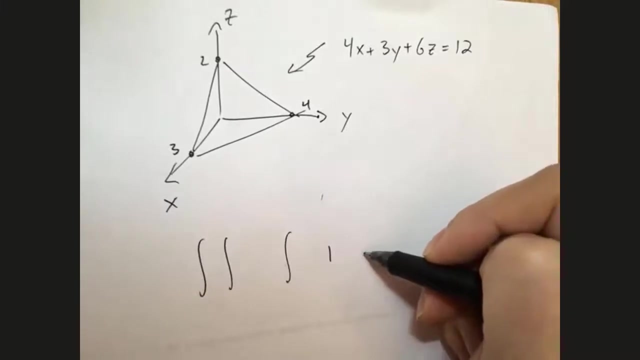 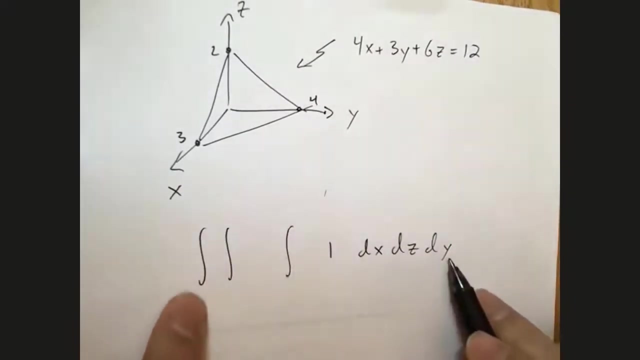 mix it up. Let's do dx dz dy. How about that? You know, I know I need to leave space here because I know how to write those functions up here, So I'm going to do. I said dx dz dy, So here I'm starting with my y. all right, So start with a y And then ask yourself: 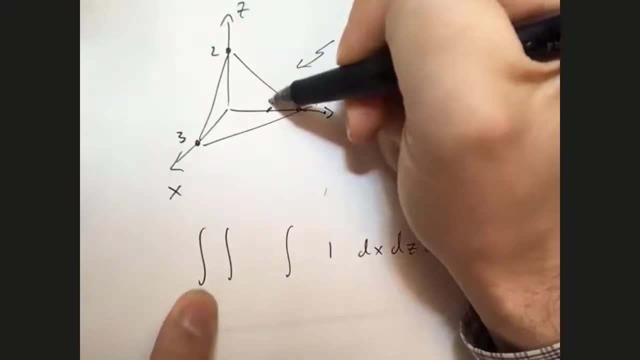 oh, what am I doing next? I'm going z, So I'm going in this direction. I'm going up in the z direction. So, for any fixed y, I'm going to go up here, I'm going to integrate with respect to z. 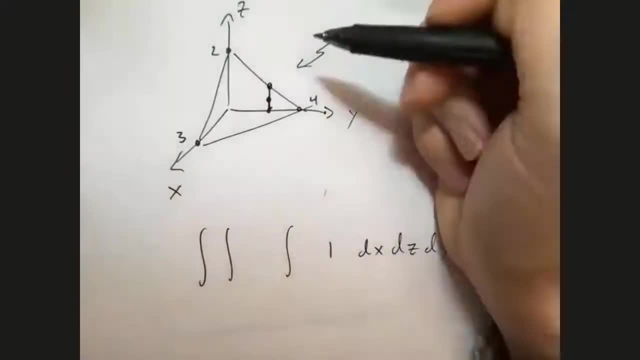 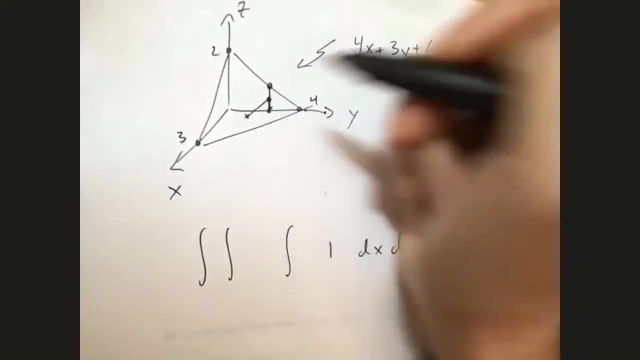 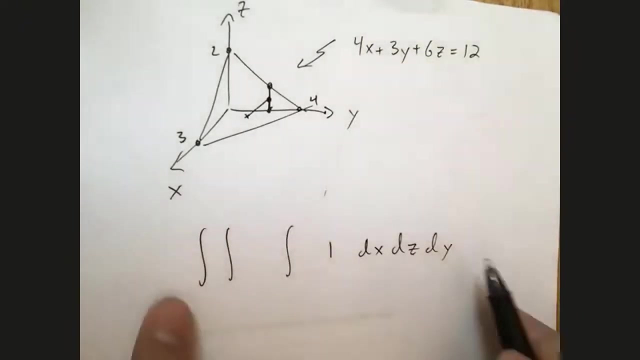 So, as I move along this line, I'm determining a y and a z. So then, for each fixed y and z, how far do I come out in the x direction until I hit this surface? That's how we're doing it this way. Okay. so what does y range from? y goes from 0 to 4.. 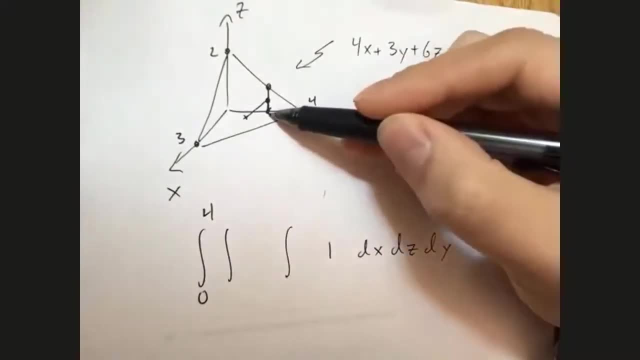 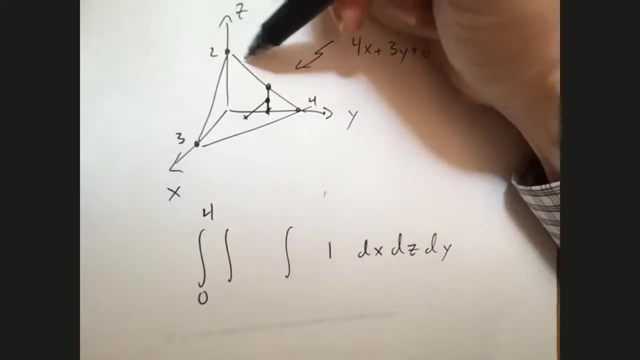 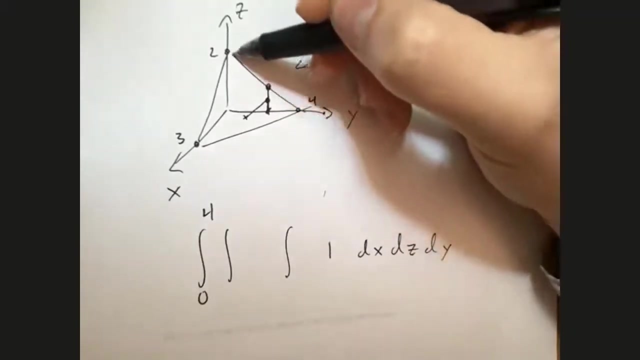 Okay, now for each y between 0 and 4, how high does z go? Well, it depends, because it depends on what y is. This is not a horizontal line, It's a diagonal line, So it depends on the value of y. I need to find this line as a function of y. Okay, so what is? 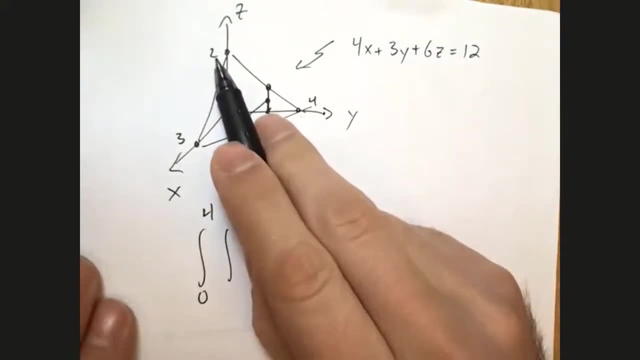 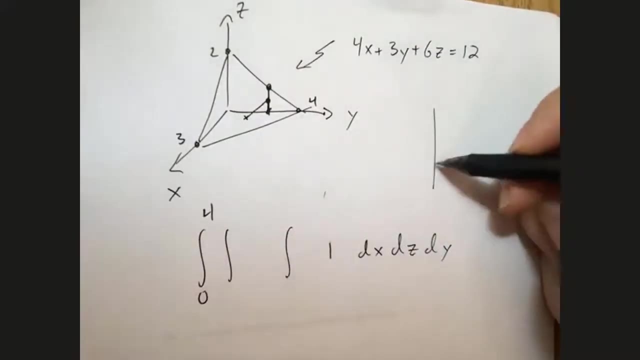 that Well, z-intercept is 2, and its slope is down 2 over 4,, so negative 1 half. So in the y-z plane, right, I'm just going to draw that line. I'm going to draw that line. I'm going to draw that line. 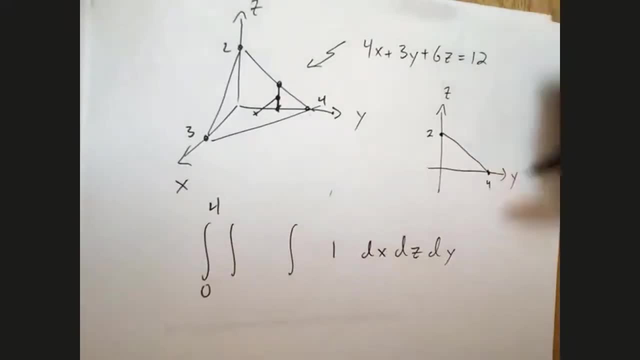 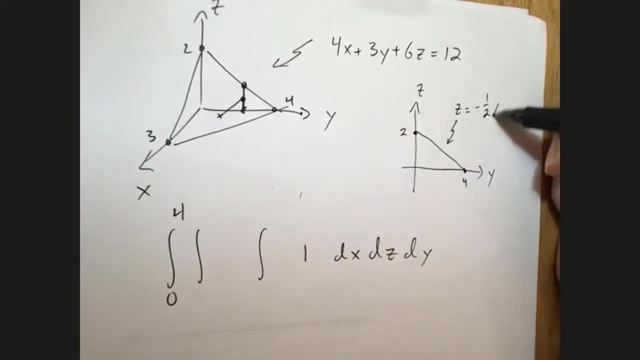 Again, it just looks like this: z is equal to negative, 1 half y plus 2.. Just mx plus b, except it's my plus b because y is the variable. So for each fixed y, that is how high I have to go. Okay, so z, let's go back down to. 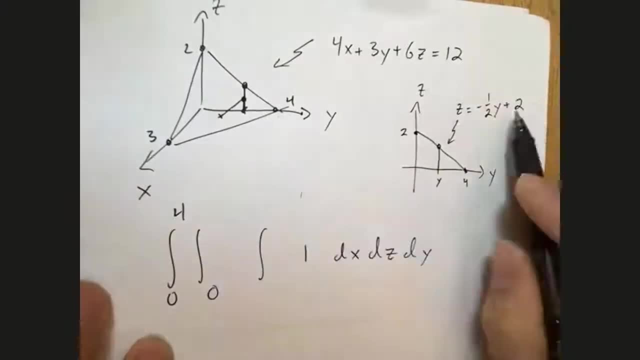 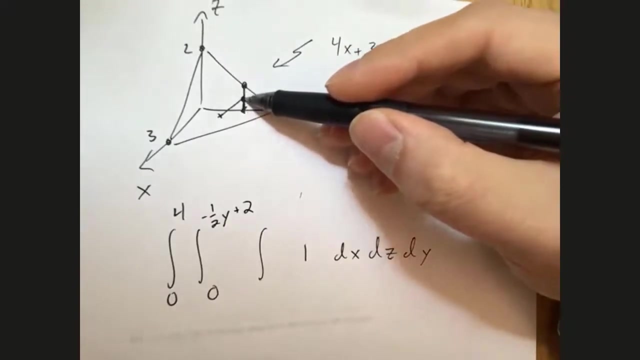 the integral z is going to go from 0 up to this high negative 1 half y plus 2.. That's moving up along this line segment in the back. So now, as I move along that line segment, I've specified both a y and a z. So now I have to ask: